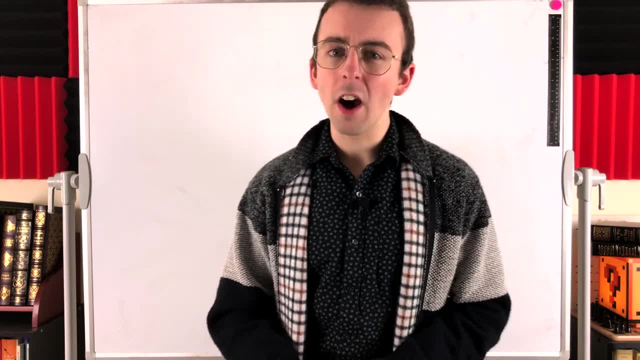 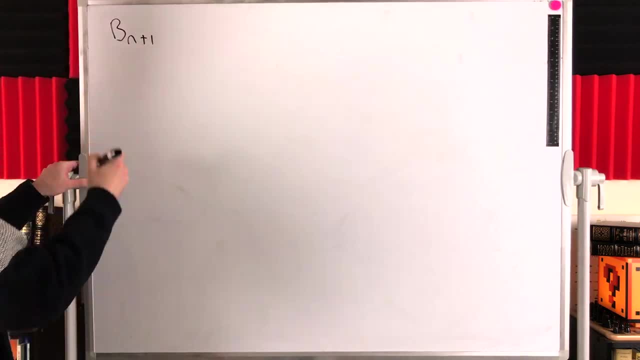 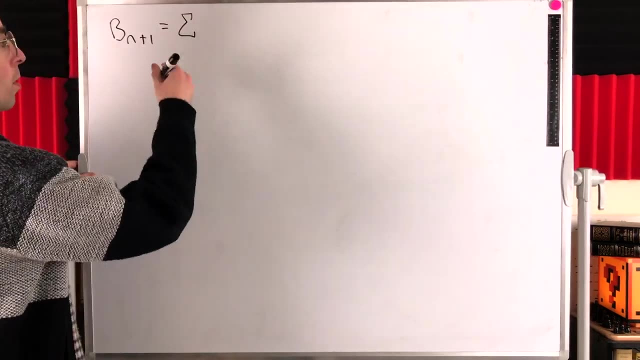 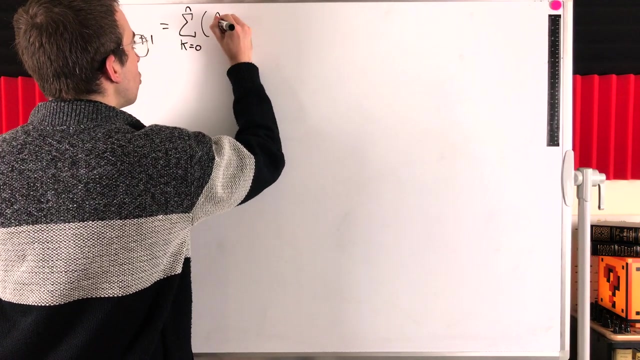 the number of partitions of a set of n objects. And in today's Wrath of Math lesson we'll be proving that to find a bell number, say bn plus 1, so the n plus 1th bell number, we can calculate this using the previous bell numbers by summing from k equals 0 to k equals n and choose k. 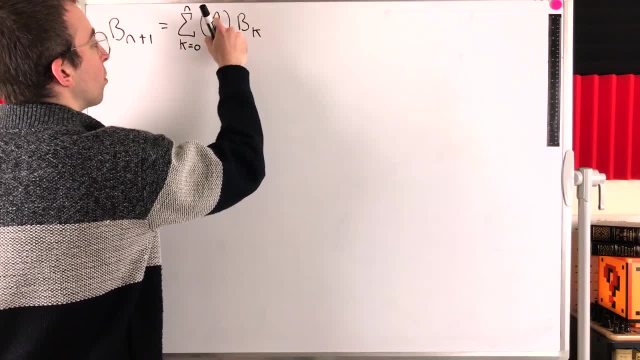 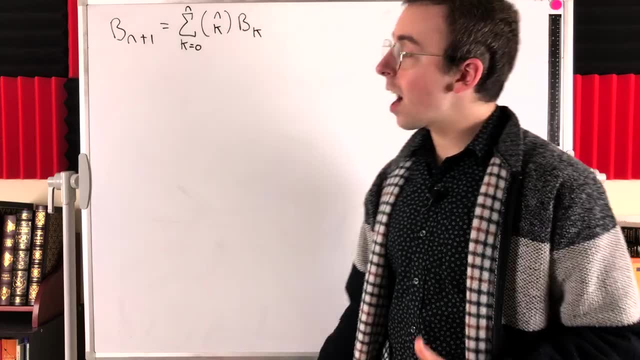 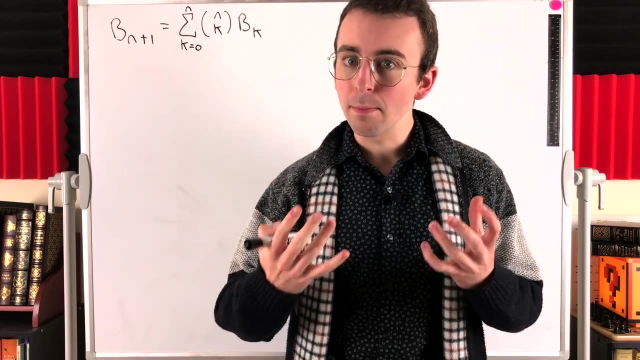 multiplied by the bell number bk. So this is the very nice recurrence relation for the bell numbers we'll be proving in today's Wrath of Math lesson One more time. remember the bell number BN, or BN plus one tells us the number of ways we can partition a set of N plus one. 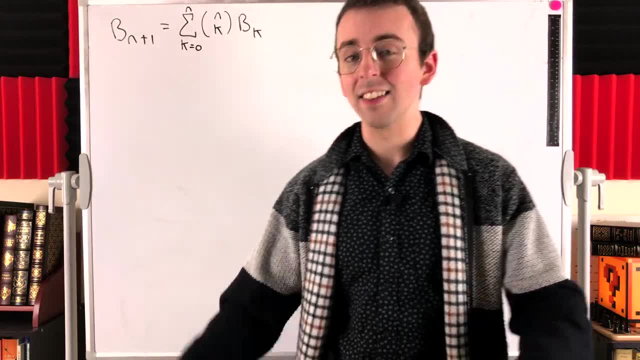 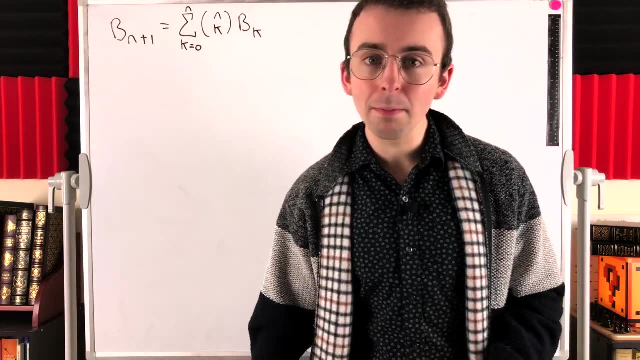 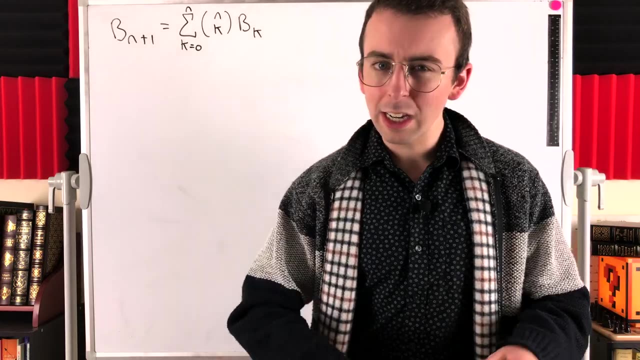 objects. That's what the bell number BN plus one is. I'll leave links in the description to previous lessons I've done introducing partitions of sets, introducing bell numbers and explaining where this recurrence relation comes from without proving it. So if, after the proof you're still not quite sure about some of the details, you'll definitely want. 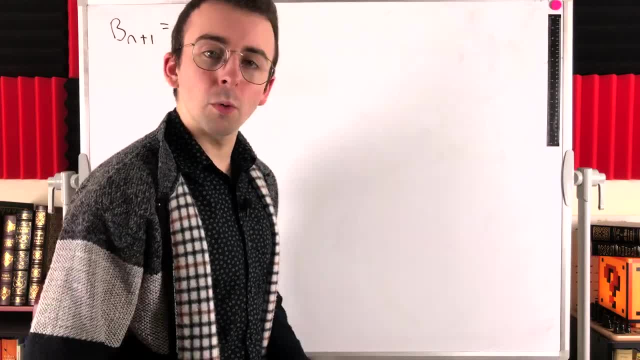 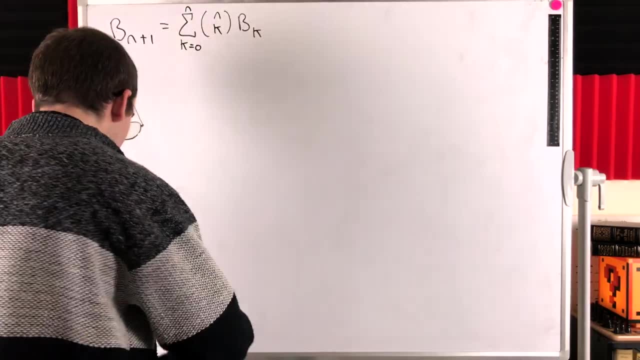 to check out some of those lessons, and you might even want to start watching some of those lessons before you watch the rest of this one. We're going to get into it, though. It's a pretty straightforward proof, all things considered, and we'll start writing it in. 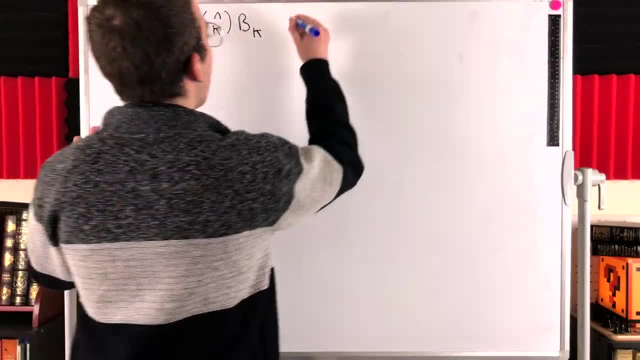 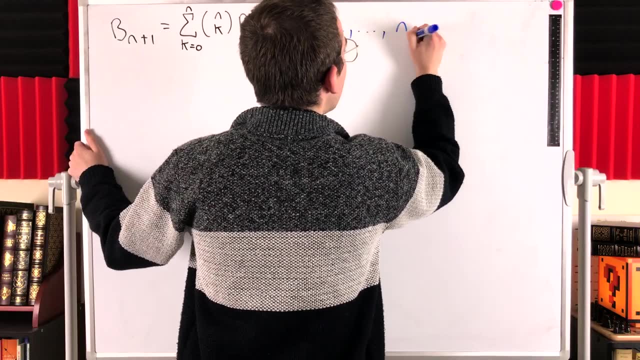 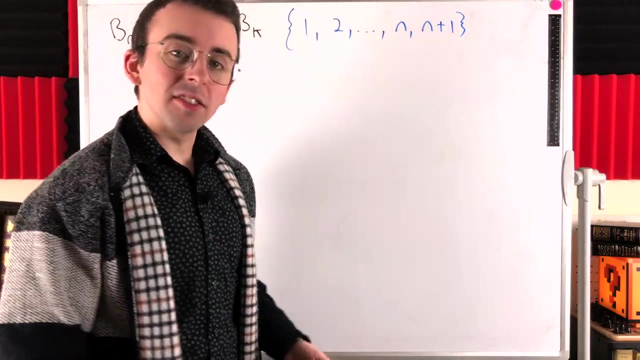 blue. So let's say we've got a set of N plus one elements which will represent, like this, a set containing one, two and so on, all the way up to some N plus one element, Of course, the actual elements in the set. 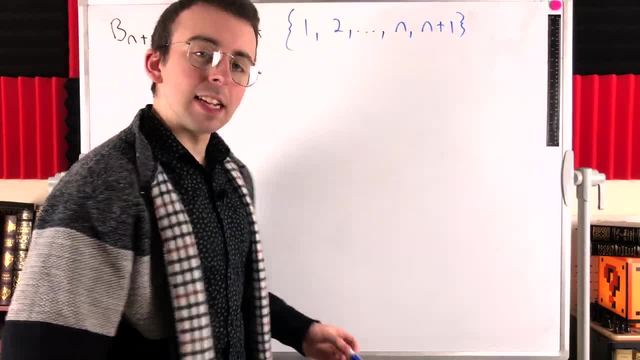 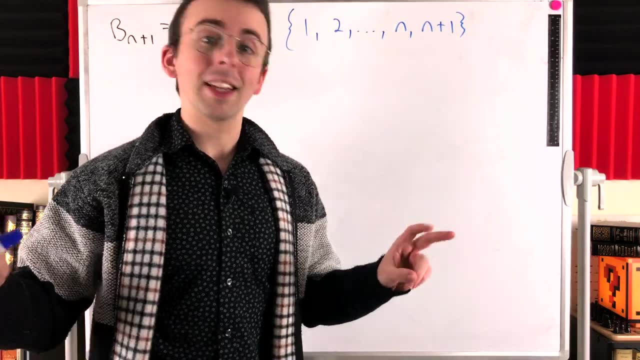 That don't matter. All that matters is the number of elements in the set. That's what's going to determine the number of ways we can partition the set. So you can think of these numbers as just labels for whatever set we happen to be partitioning. And let me redraw. 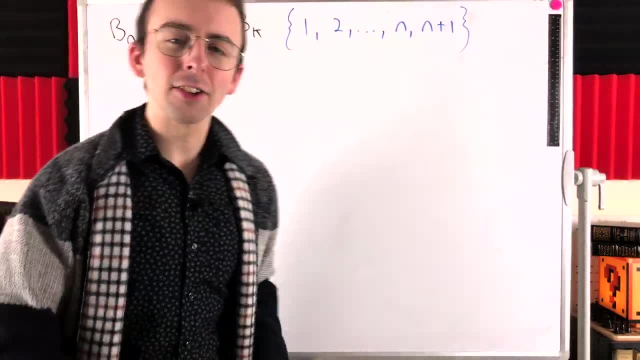 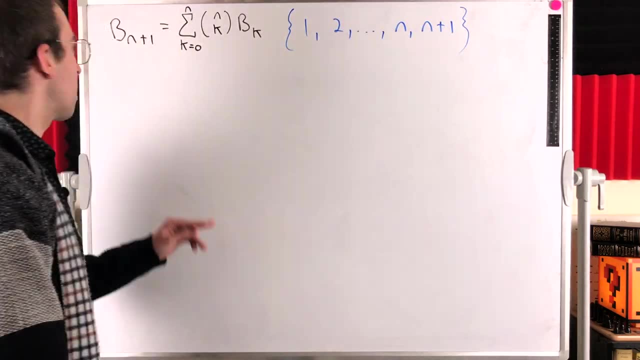 the bracket at the end, because I accidentally drew it really small. That looks a little nicer. So we're trying to find the number of ways we can partition this generic set of N plus one objects, That's the bell number, BN plus one. So we're going to go ahead and do that. So we're going to go ahead and do that. So we're. 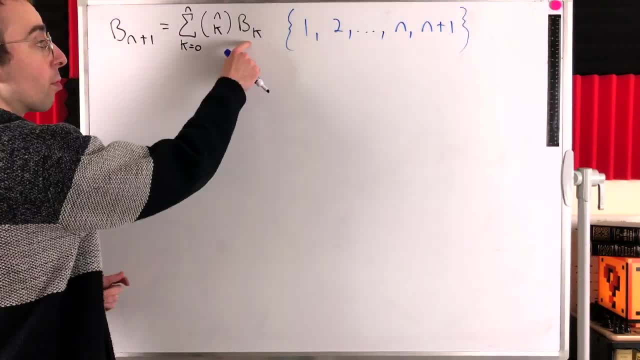 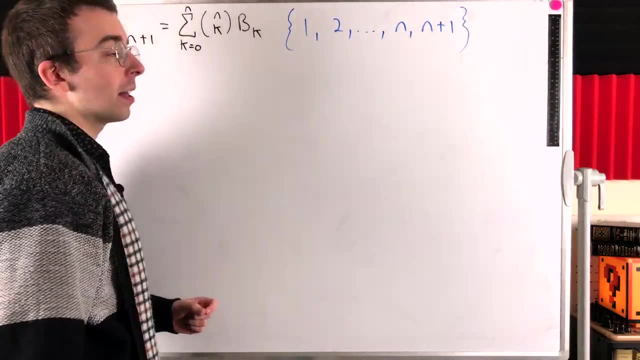 going to go ahead and do that Now, in order to figure this out in a way that uses the previous Bell numbers. naturally, we're going to have to find a way to consider some smaller sets where those other Bell members are going to come in handy. So how could we? 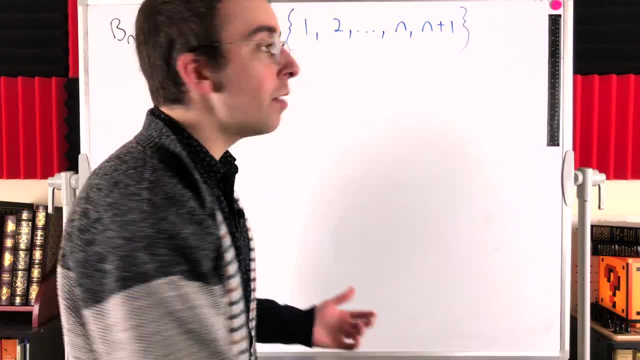 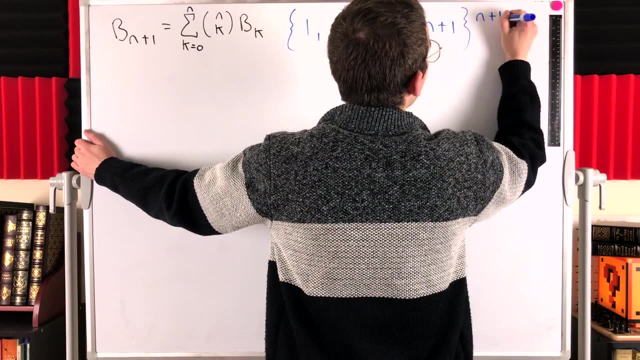 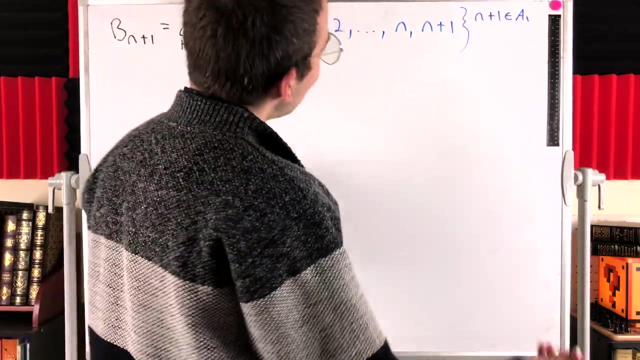 do that. Well, we know, if we have just some given partition of this set of N plus one objects, certainly the last object there, N plus one, has to be an element of some part of the partition. Call that part a1.. And let's say that the cardinality of this part of the partition that contains n plus 1,. 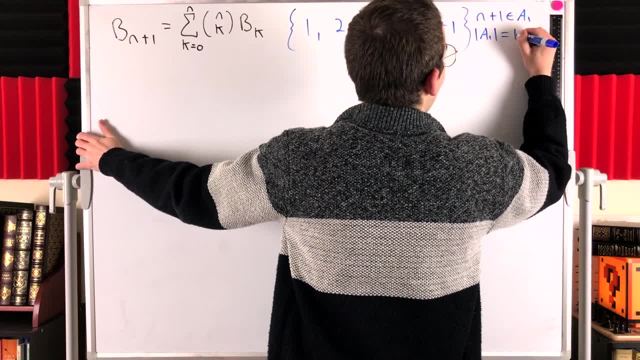 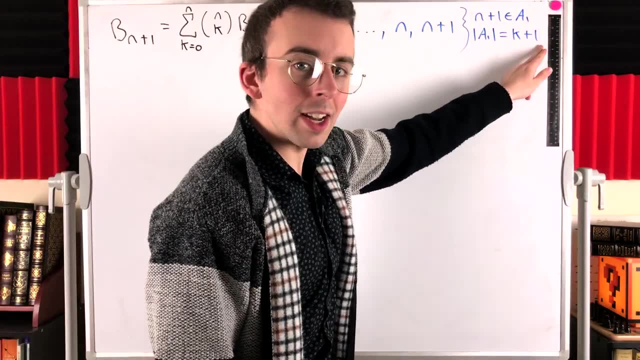 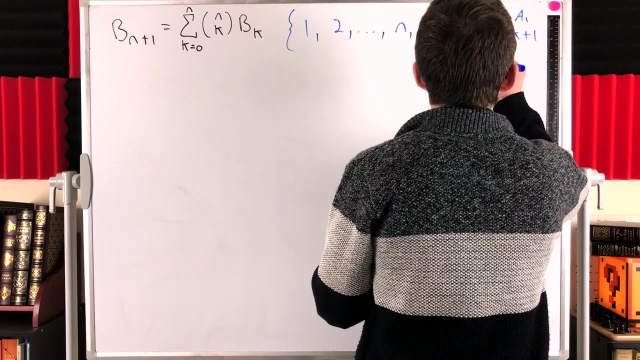 the cardinality of this part of the partition. let's just say it's equal to k plus 1.. Thus it contains the object n plus 1, and it contains k other objects as well. What are the possible values of k? Well, k could be as small as 0, meaning that the only object a1 contains 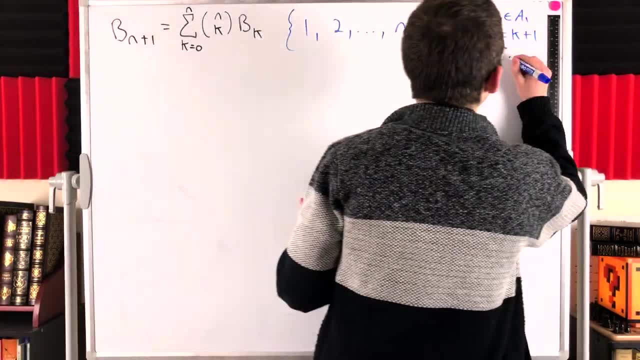 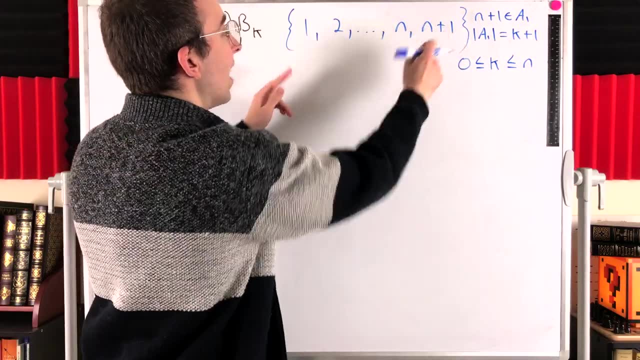 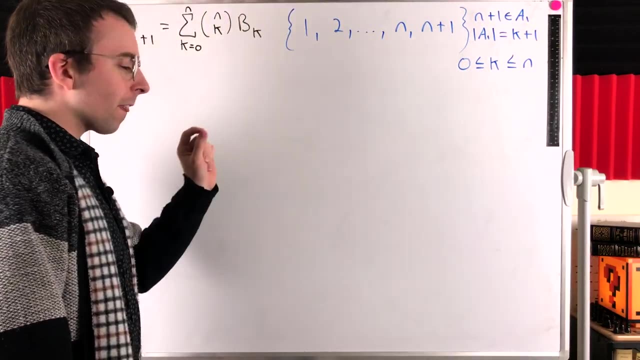 is that n plus 1th object, Or k, could be as big as n, meaning that a1 contains n plus 1. objects, as in all objects of the set have been put into the same part. That's another possible partition. Okay, so there are still some elements unaccounted for, right. 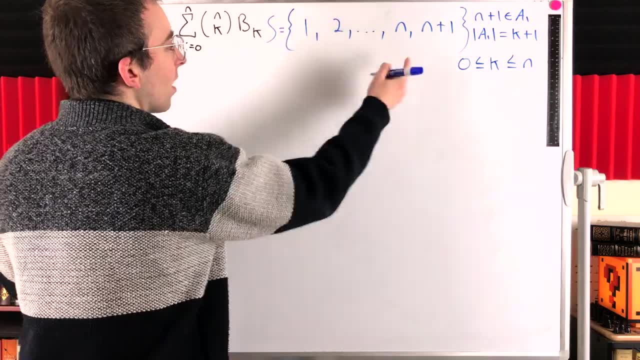 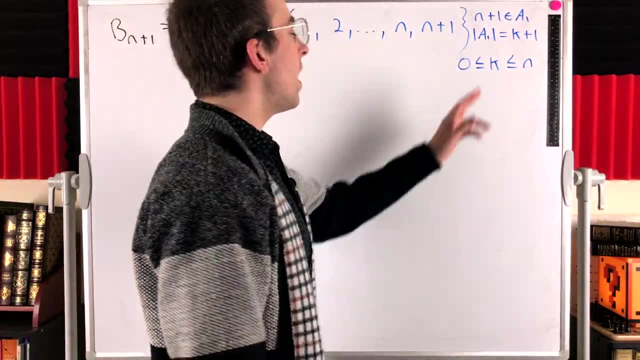 The total set. here we'll call this set s. it's got a total of n plus 1 objects. And now we're saying if we partition it, one of those parts- say a1, includes the element n plus 1.. So let's. 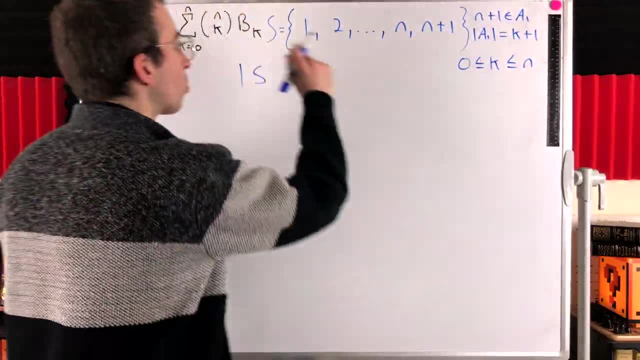 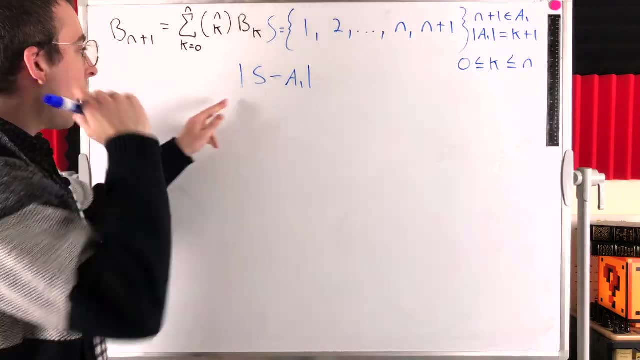 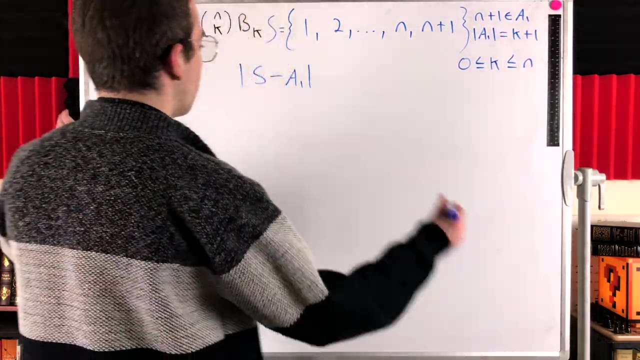 say we get rid of this part a1. Suppose we subtract it from the set s and we consider the set s minus that part a1, how many elements are left? How many elements are outside of the set s? How many elements are inside of this part that contains n plus 1? Well, the set s has n plus 1. 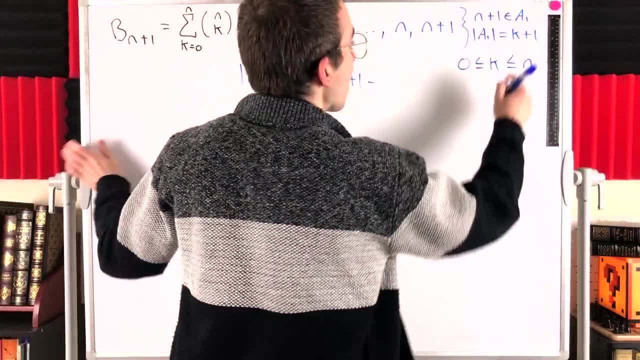 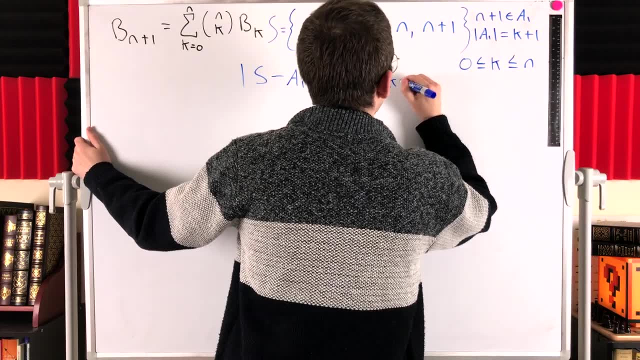 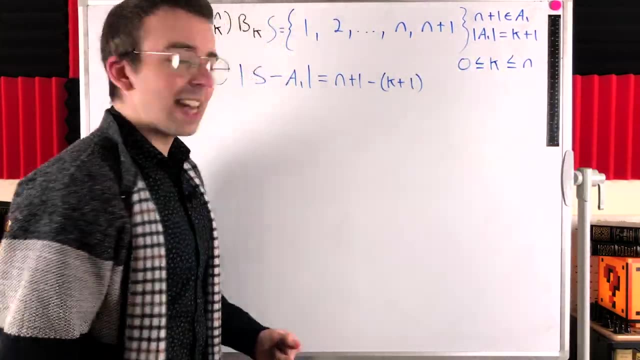 elements total and we're removing k plus 1 of them because we're removing all of the elements of a1. So it's just n plus 1 minus k plus 1.. That's the number of elements left that we have to partition. We know that k plus 1 of the elements have been put in a1, and we have n plus 1 minus k. 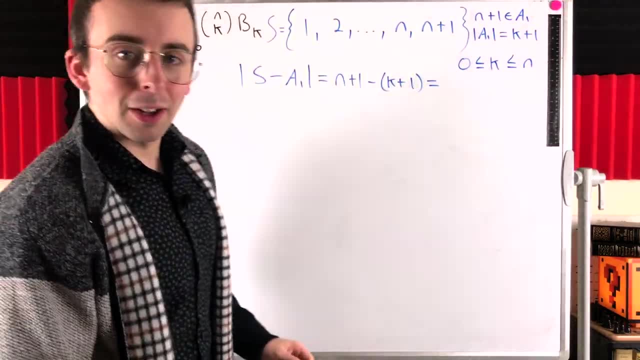 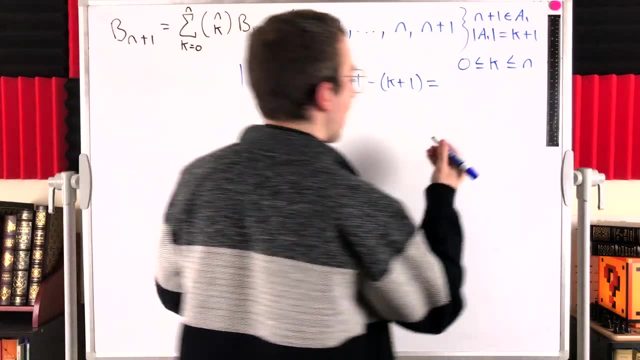 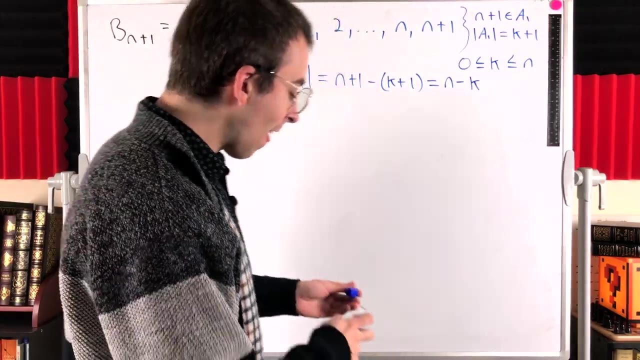 plus 1 elements left. What is n plus 1 minus k plus 1?? Well, it's just n minus k plus 1 minus 1, which is just n minus k. So there are n minus k objects left to partition outside of our part a1.. So what we've done here? 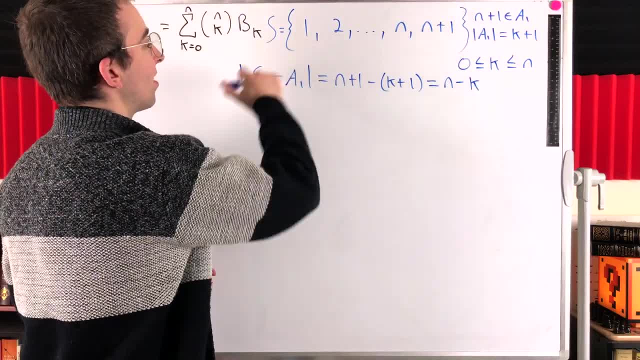 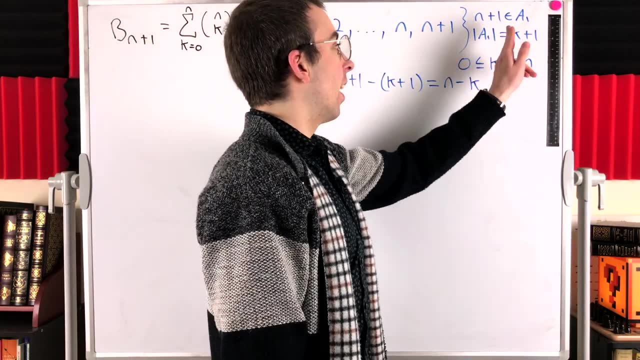 is sort of split the partition of our set s into two sections that we're considering. We've got our part a1 that contains k plus 1 objects, including n plus 1. And then we've got our n minus k objects left to partition outside of our part a1. So what we've done here is sort of split. 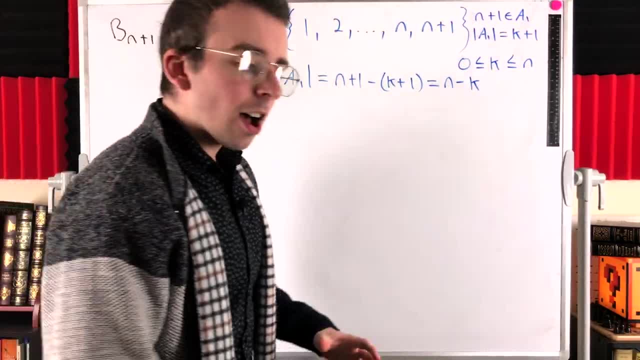 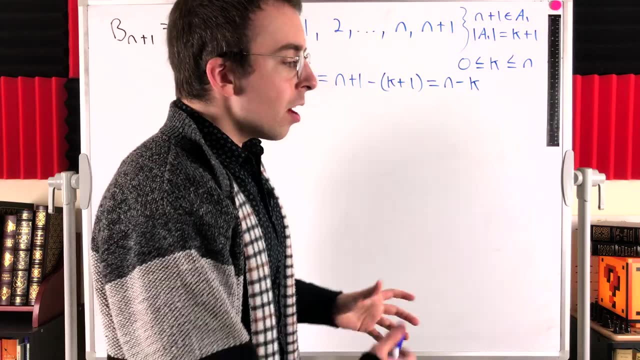 the partition of our set s into two sections that we're considering. We've got our part a1 and then we've got the other n minus k objects that still need to be partitioned. So let's count the number of ways that these two things could happen For some given value of k. how many different parts? 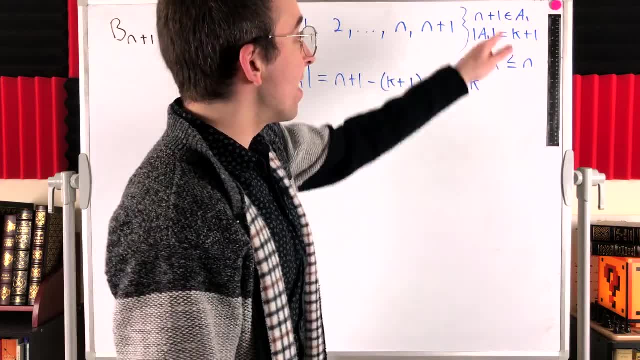 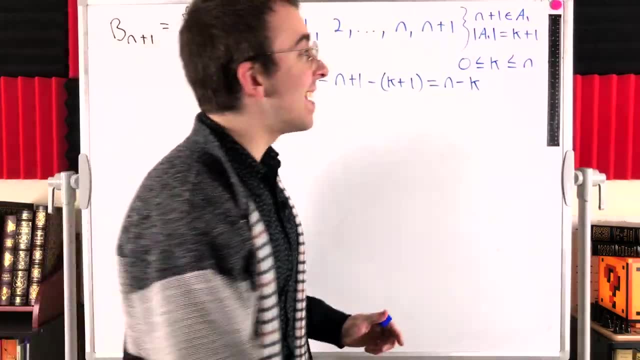 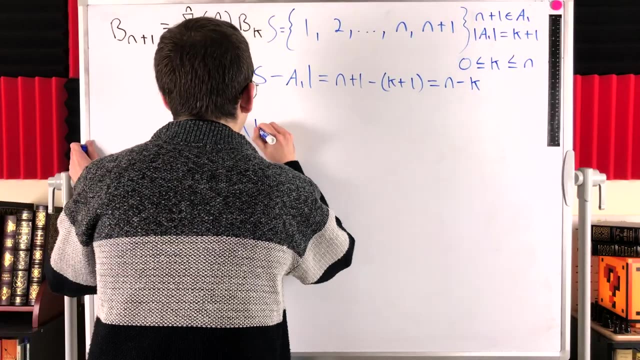 are there containing k plus 1 elements that also contains the element n plus 1?? Well, if we're guaranteeing that the part contains the element n plus 1, then we just have k elements left to pick To put in the part a1. So we've got to choose k elements. How many elements do we have to choose? 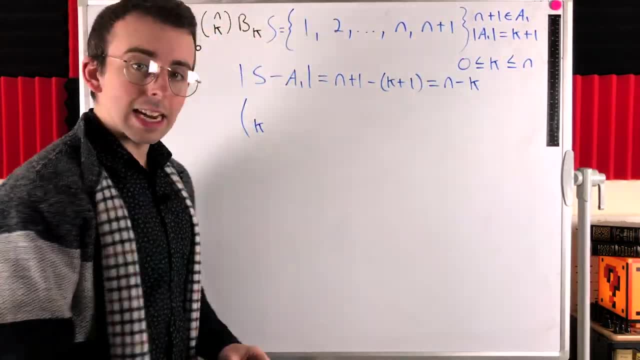 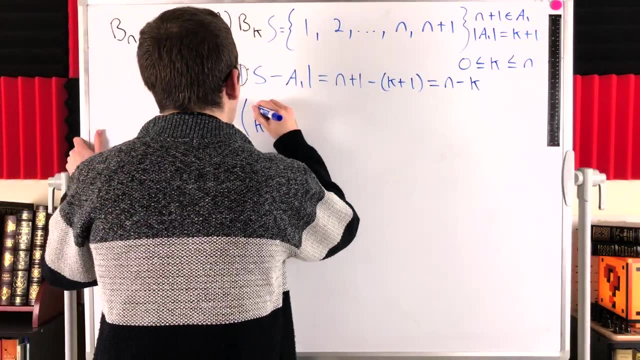 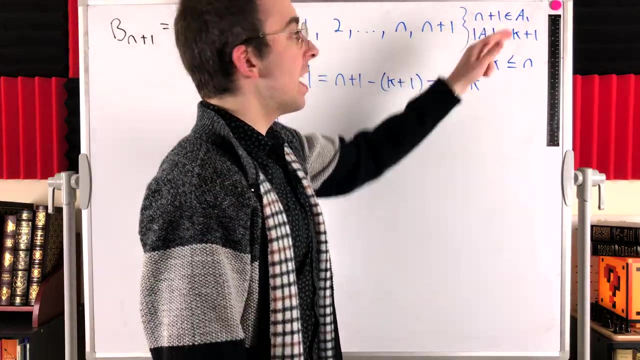 from. Well, we've already put n plus 1 in the part a1. So we have all of the other elements left to choose from, All n other elements. So there are n choose k total parts of cardinality, k plus 1, that we could put the element n plus 1 into Now for every one of those possible. 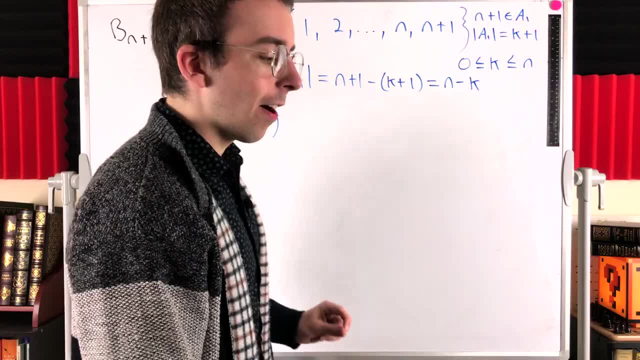 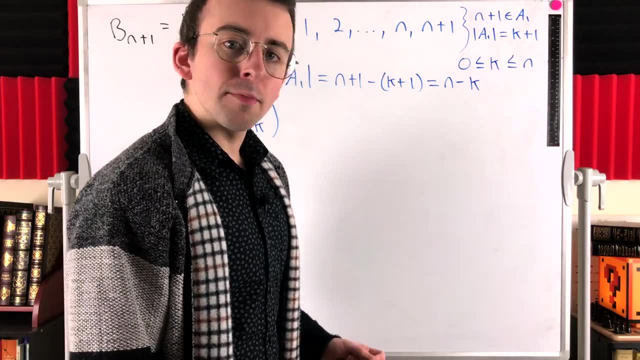 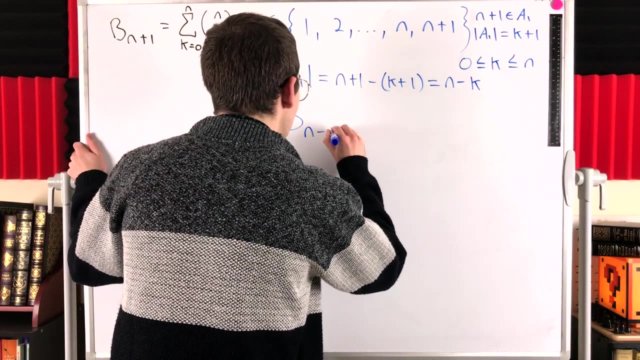 parts a1, that n plus 1 could belong to. how many ways could we partition the remaining n minus k elements? Well, the number of partitions on n minus k elements is a bell number. It's the bell number b, n minus k. And now look at this. looks like we're starting to get somewhere. So what? 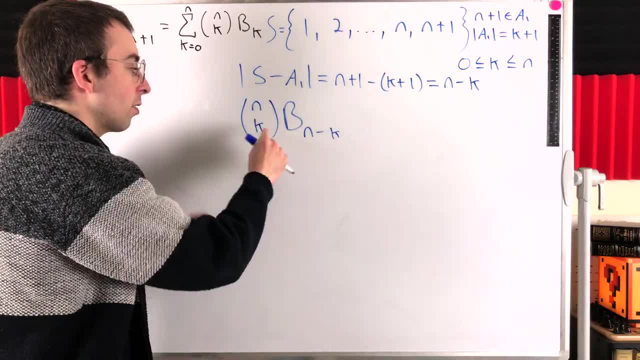 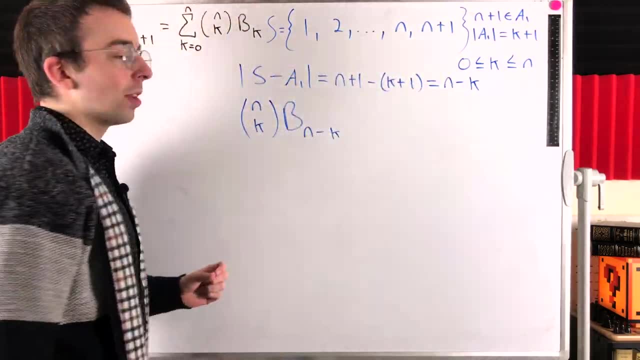 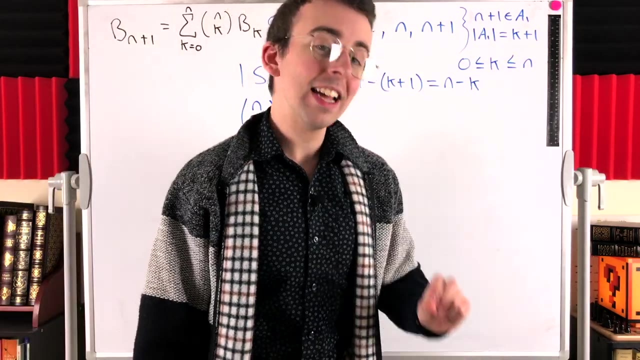 we've just gone over this expression. this gives us, for a given value of k. this gives us the number of partitions of this set on n plus one objects where n plus one belongs to a part that has k plus one: total objects. That's what this expression gives us. However, we know that k can be as small. 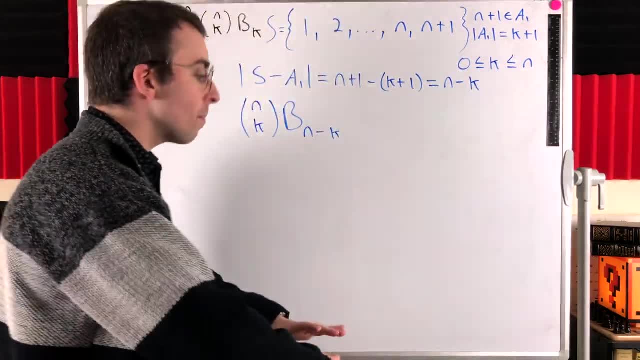 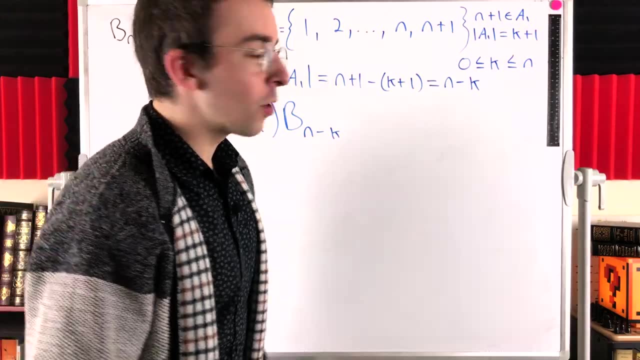 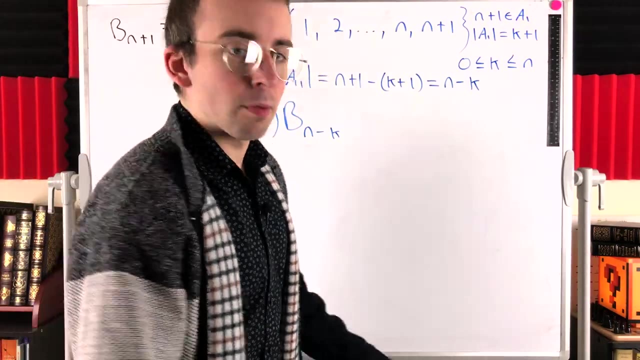 as zero or as big as n. So to count up all possible partitions of this set, all we have to do is add this expression to itself over and over for all possible values of k, just like that. That's the vast majority of the logic in the proof, If you understand me up to now. 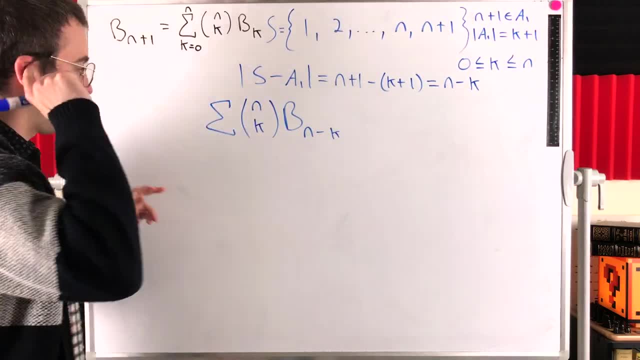 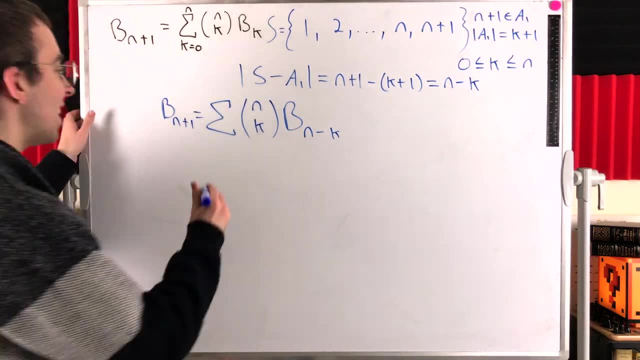 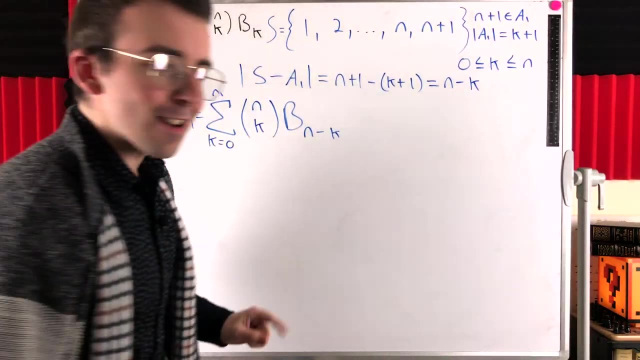 I think we will be golden. Now let's finish things off. So all we have to do to find the bell number b n plus one, all we have to do is take this sum from k equals zero- to the maximum possible value of k, which is n of n. choose k times the bell number b n minus k. That's how we find that next. 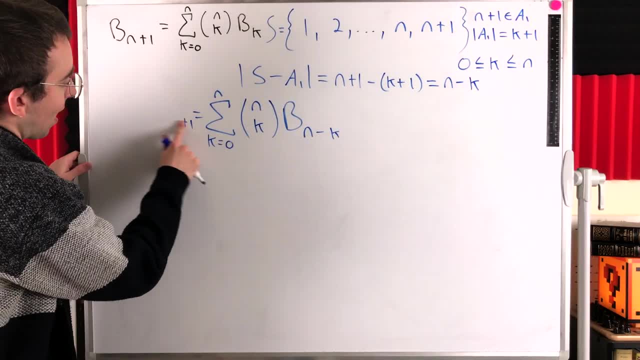 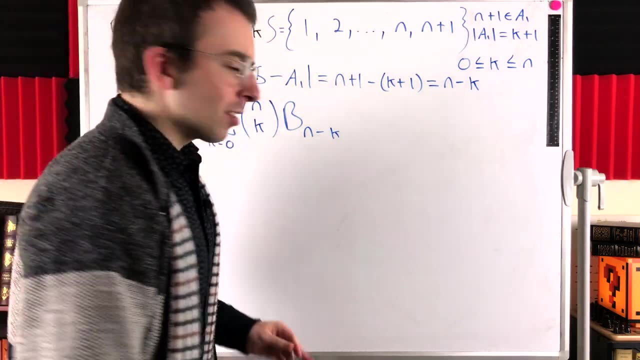 bell number b n plus one. And let me just rewrite that b n plus one because it's looking kind of crooked. So this is our expression for b n plus one. Okay, so what's going on here? This doesn't look quite. 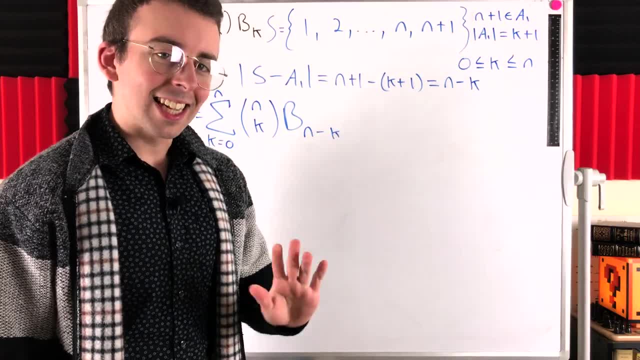 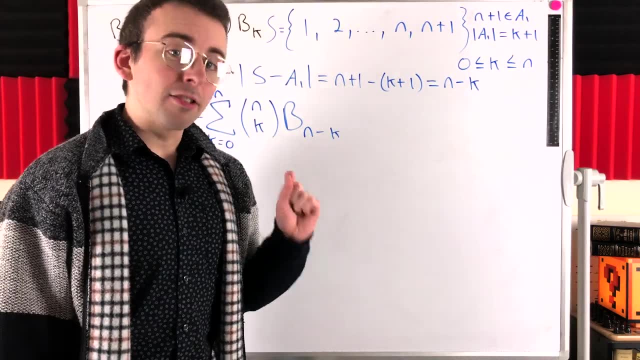 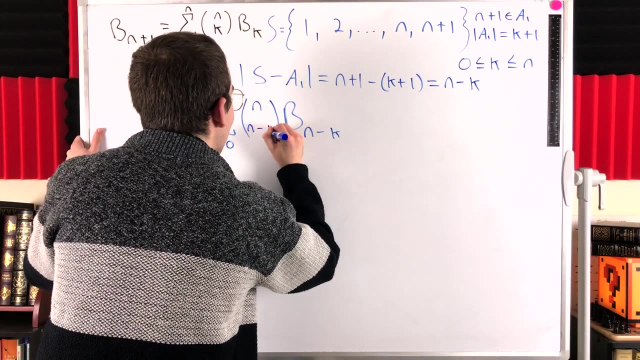 like that. It looks pretty close, but not quite. Well, let's make it work. So look at this. We've got a factor, a binomial coefficient, here, n choose k. By the symmetric property of binomial coefficients, n choose k is the same as n choose n. 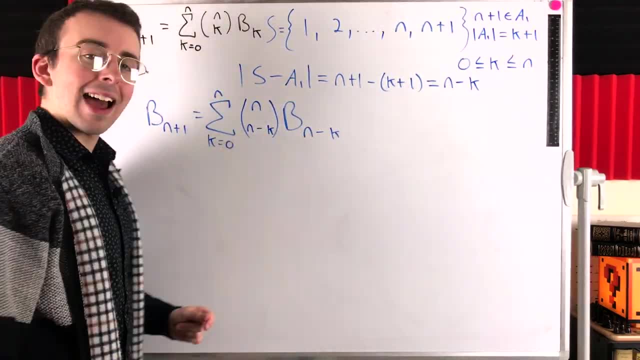 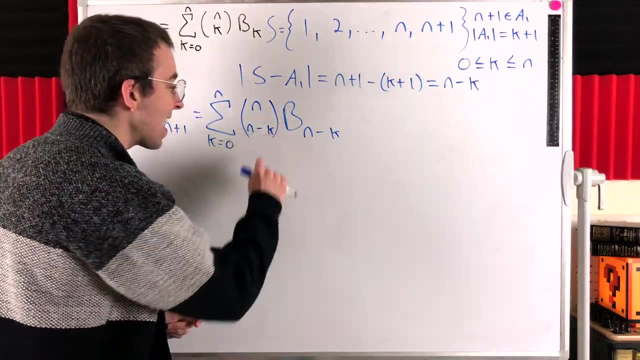 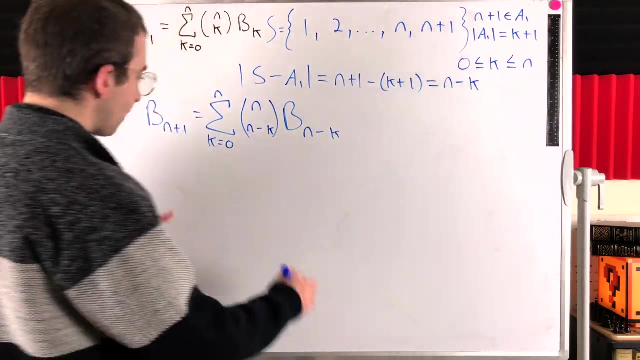 minus k. I'll leave a link in the description to a proof of that fact. The basic idea is that n choose n minus k is the same as picking k elements to not choose, which is, of course, n choose k. Again, there's a link to a proof of that down in the description. Okay, so then what is this sum? 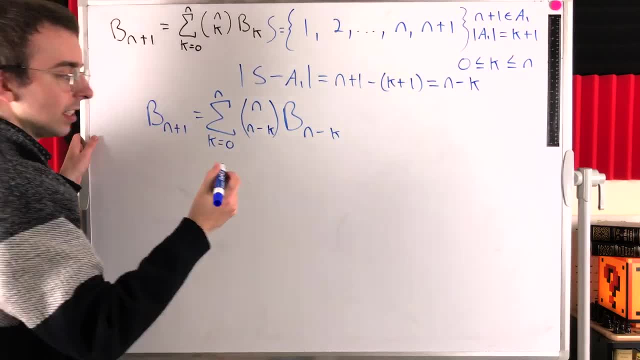 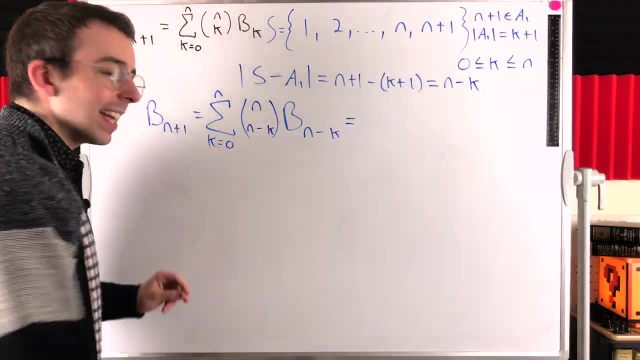 equal to. Can we show that this is equal to this? Well, indeed, we can. we really don't have much work left to do here. Let's just write out what the terms of this sum look like. We start at k equals zero. So that's going to be n, choose n. starting at k equals zero. 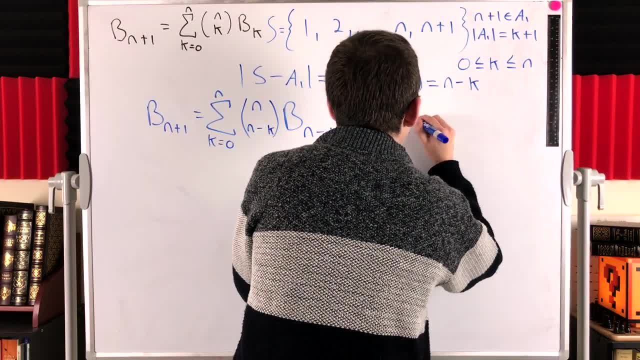 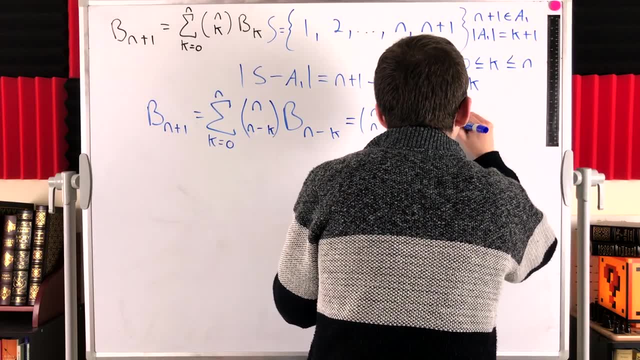 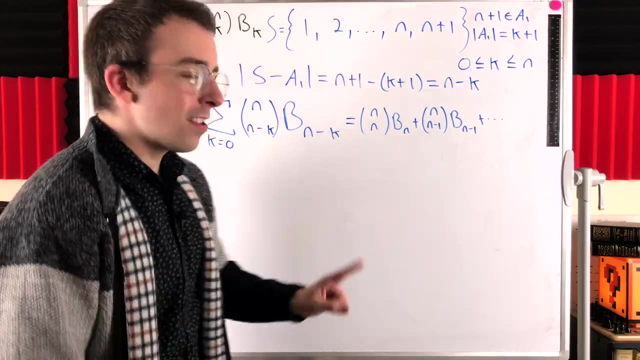 we're going to have n choose n times b? n, then k is going to go up to one and we'll have n choose n minus one multiplied by the bell number b n minus one, And it's going to continue in this way, with this and this going down by one in each term going down by one. Finally, I wish I had a. 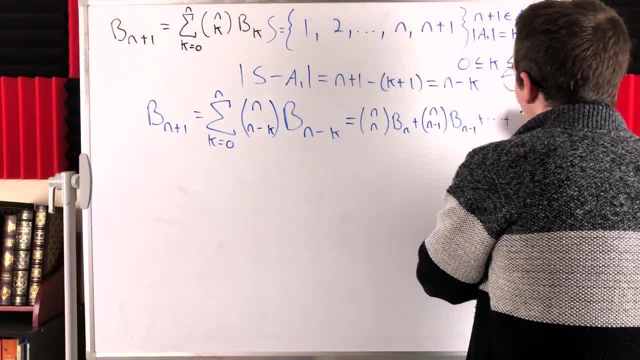 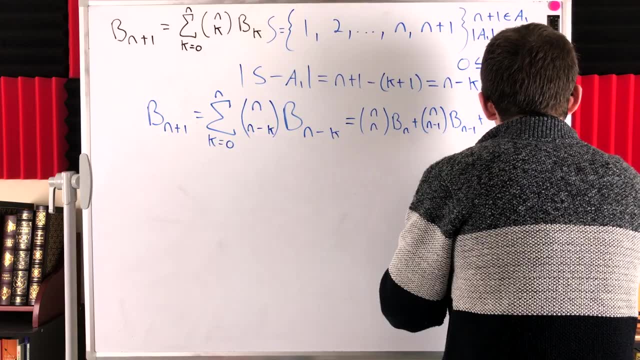 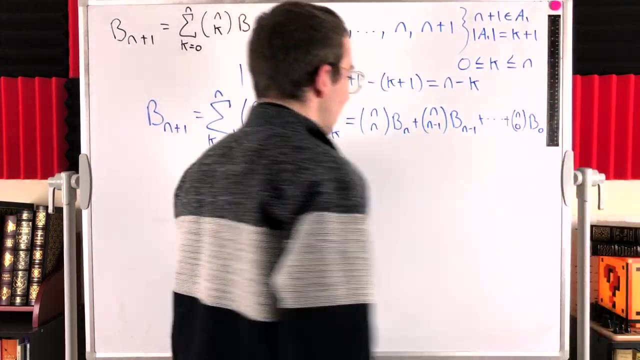 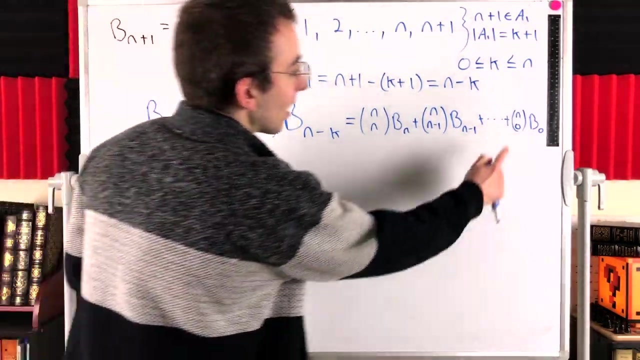 little more room here, but it's going to end with the final term at k equals n. that's going to be n choose zero, n choose zero multiplied by the bell number b zero. So look at this: This is the sum we want, just written in reverse order. we've got n choose zero times b zero. that's the first. 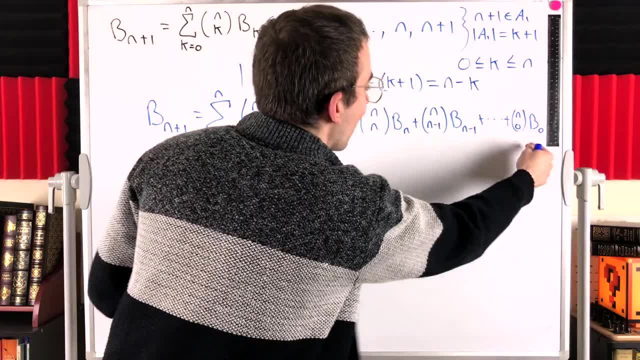 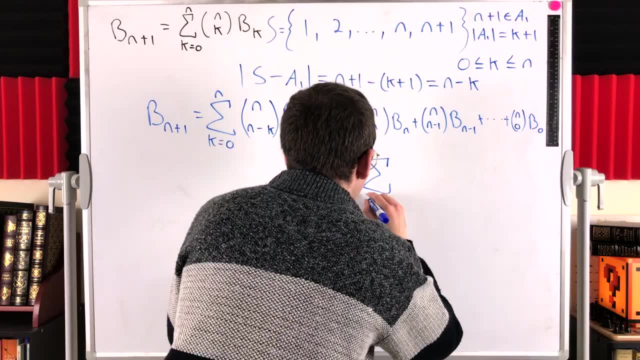 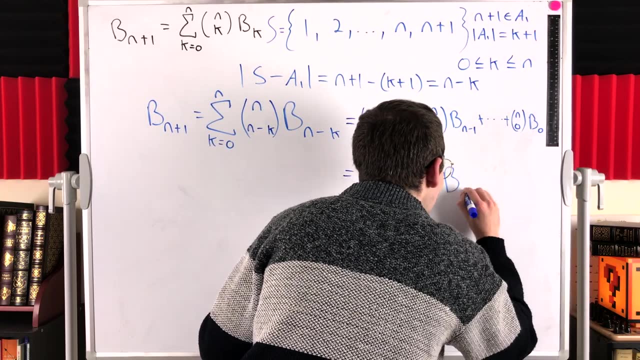 term of this sum, And then these are going up by one this way each term. So what I'm saying is this is the exact same as this sum. the sum from k equals zero to k equals n of n. choose k times the bell number b- k. 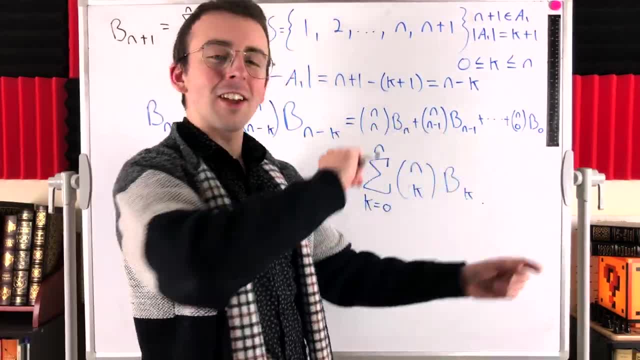 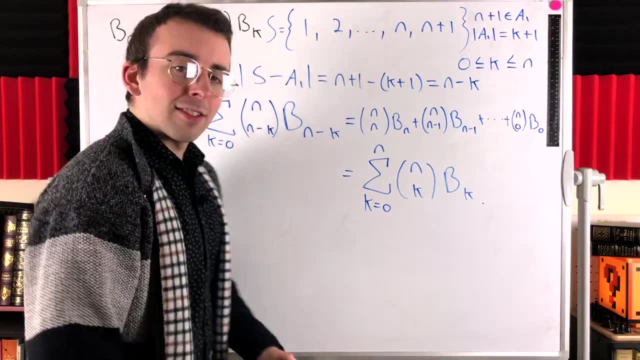 Just written in reverse order And of course it's just a finite sum. So flipping the order that we're adding the terms in doesn't change anything at all, Because look, you know what's the first term of this sum going to be. 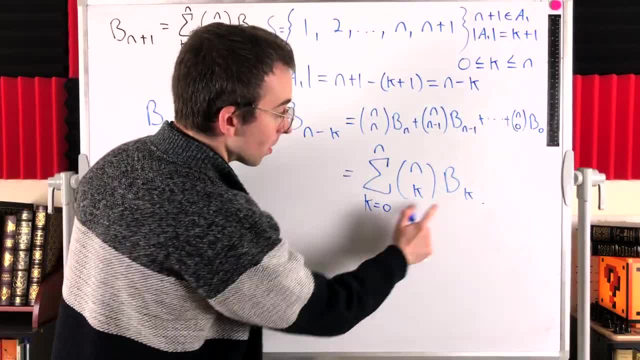 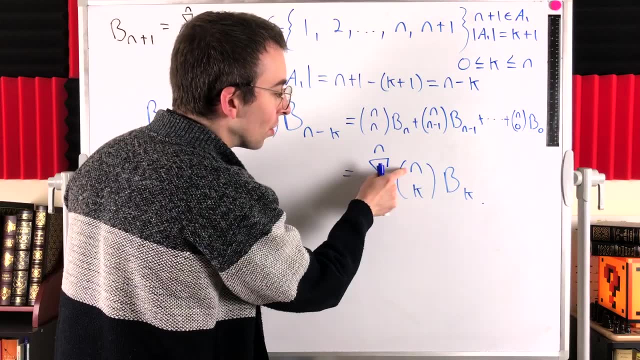 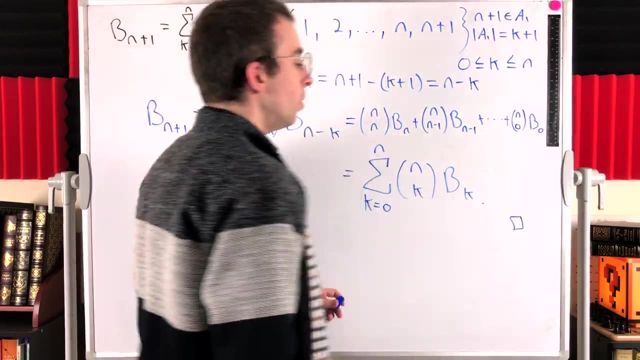 It's when k equals zero. So we have n choose zero times b zero And they're just going to keep incrementing up by one until we get to the last term where k equals n will have n choose n times the bell number b- n. That's the proof. All right, who could have taken a few more breaths during that proof? 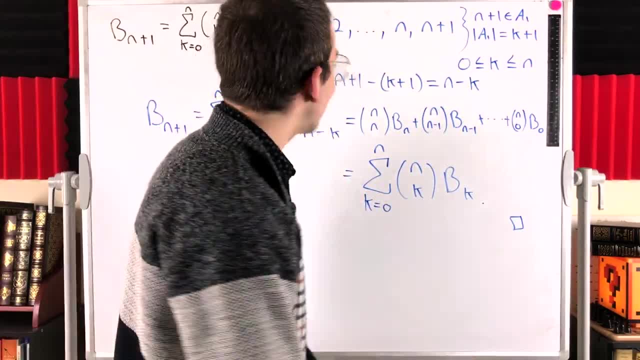 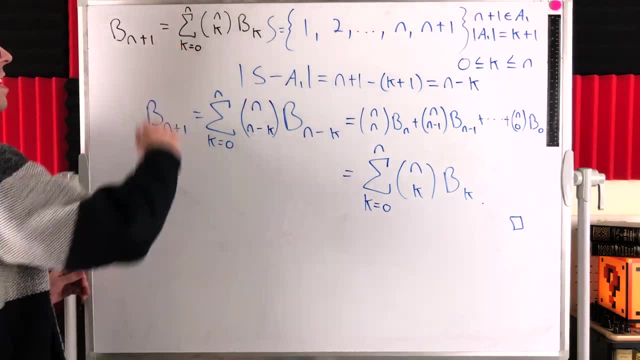 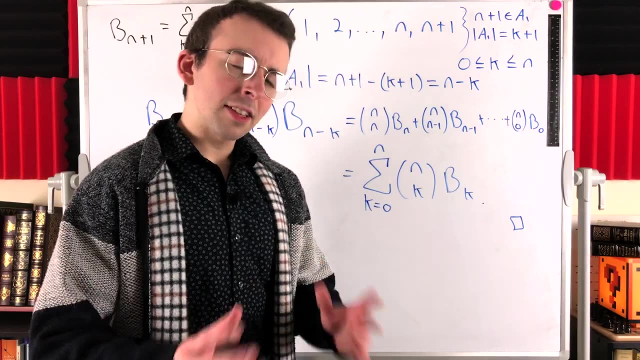 Hope that explanation was clear. So that's how we prove the recurrence relation for the bell numbers. to find the bell number b n plus one, all we have to do is take the sum from k equals zero to k equals n of n. choose k times the bell number bk. Now let's just 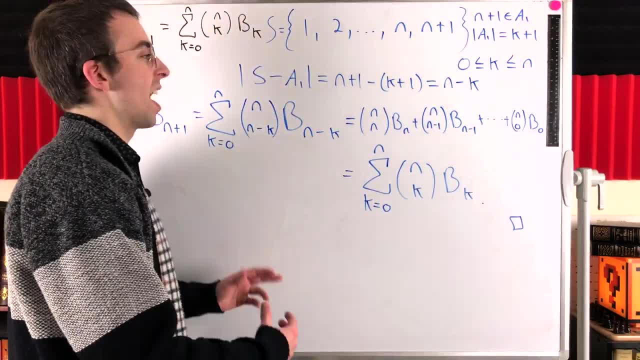 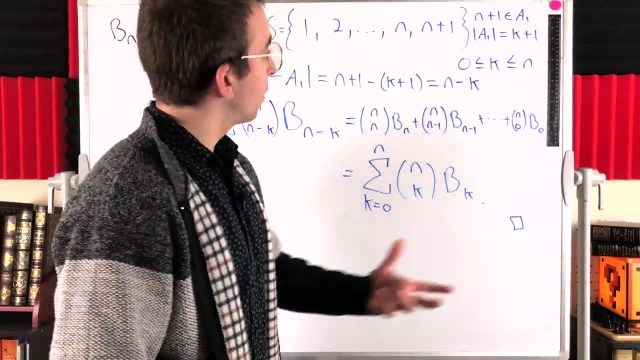 go over what I think is the trickiest part of this proof one more time where we go, you know from here, talking about our arbitrary partition to this sort of expression, the logic is that n plus first element, So this element, n plus one In any partition of this. 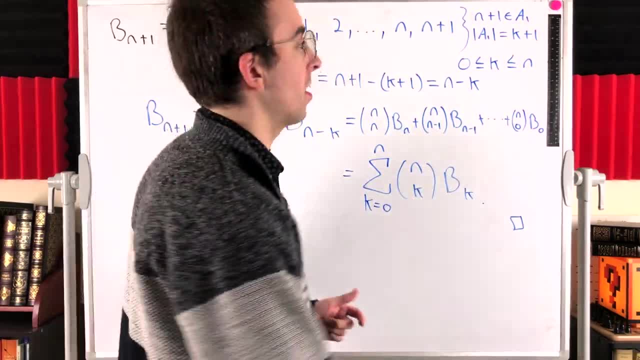 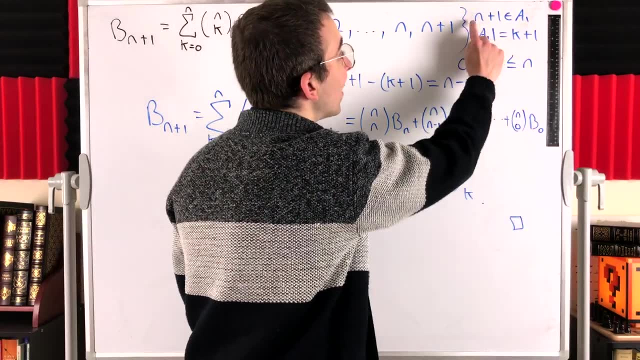 set n plus one has to be in some part of the partition. We call it the first element. So is clearly this null sign of the proposition. We call it n plus one. but if we take that we call that part a1.. Suppose a1 has k plus 1 elements. thus it has our guaranteed element n.